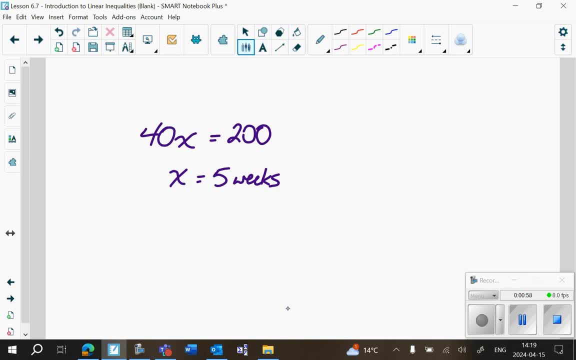 save $200?. How many weeks would she have to save to have at least $200?? Yep, So how many weeks did she? the first question was: how many weeks did she have to save to have $200?? The second question is slightly different: How many weeks does she have to save to have? 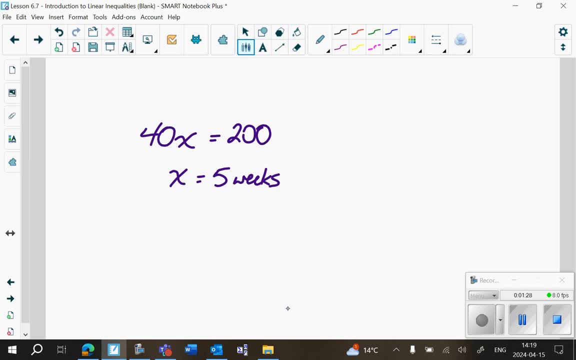 at least $200?. How would you answer it, though? Like would you just say five, Or how would you phrase it? She would need at least five weeks to save $200.. Precisely, Do you see how there's more than one answer in that situation? It could. 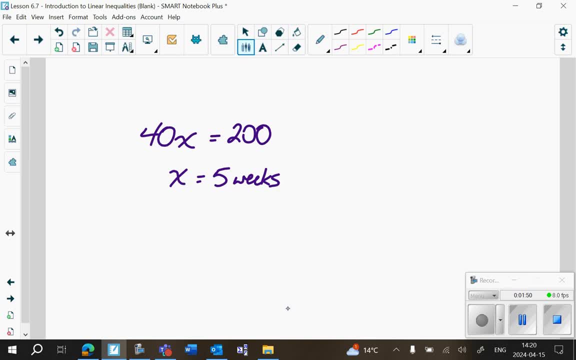 be five, it could be six, it could be seven, it could be eight, whatever There's more than one answer. okay, What if I said: how many weeks does she have to save to have $200 or less? Is there just? 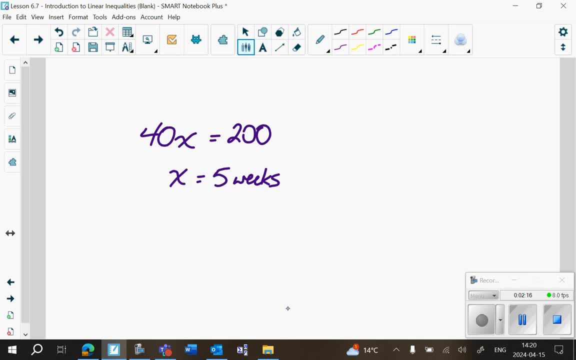 one answer or is there more than one answer? How many weeks would she have to save to have $200 or less? She would have to save Right. So would four be an answer? Yeah, Three, two, one, of course, Again there's. 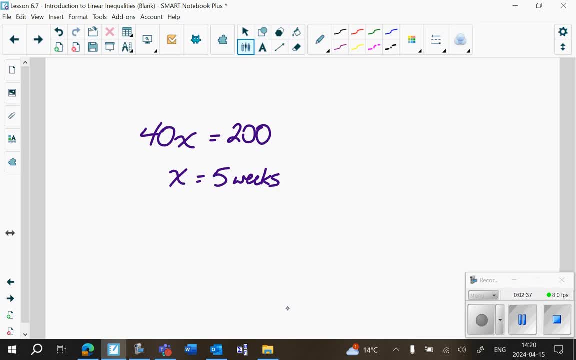 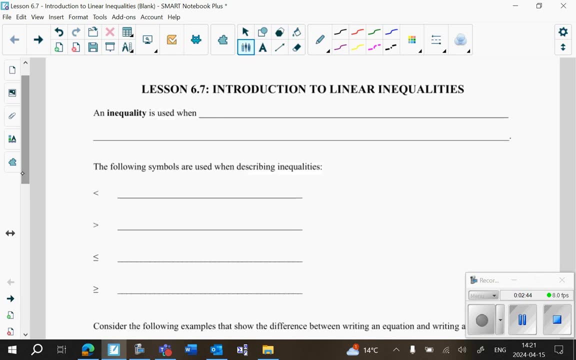 a whole range of answers. So that's something slightly different, And we call those things inequalities, So we use an inequality when we want to describe a situation where there's more than one answer. Okay, So we want. Okay, Thank you. 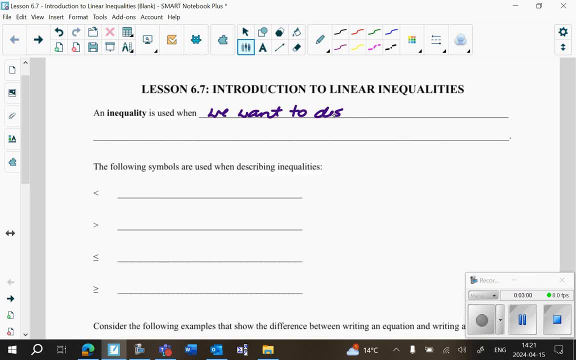 Okay, where? Yeah, okay, Okay. one could use something with that word to follow, or you could probably again think of it as an assorted solution. Okay, Okay, Sorry, There's more than one. Okay. 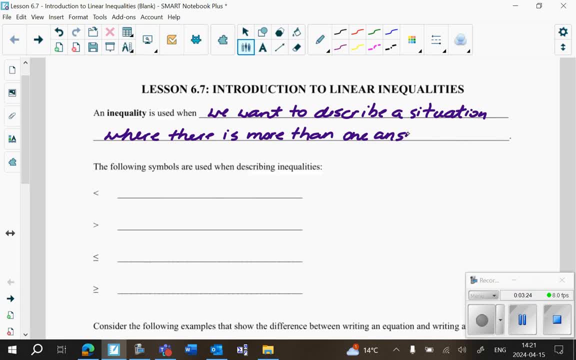 Okay, Okay, Another possibility, Another problem, Okay, A tool that could also be transformative, right, Okay? well, how do we do that? well, with equations, the symbol that we use are two horizontal bars. that mean equals, that means one answer, but if we want to show more than one answer, we use four different. 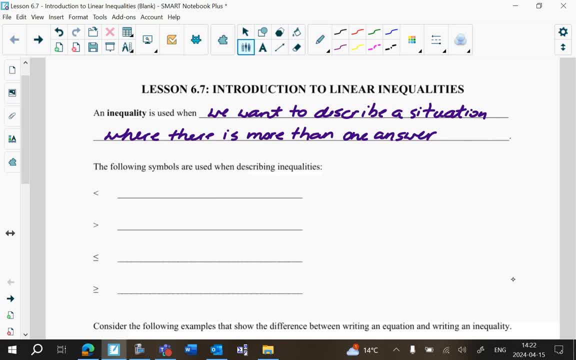 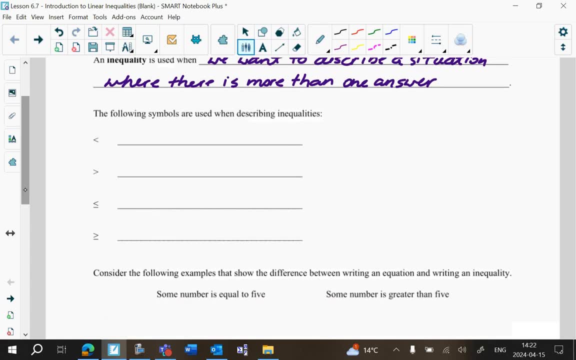 inequality symbols, two of which you should have seen already. do we remember which one equals or which one is which? do remember when the point is going to the left. remember we always read an equation like we read an English sentence, from left to right. anyway, you want to take a shot? 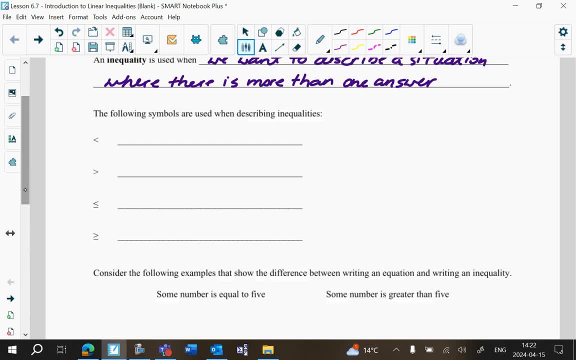 you got a 50-50 shot. less than the point is pointing to the left. it's pointing to the smaller number. if the gap, that's a wide part, is pointing to the left, that's greater than some of you may have seen these symbols before, or 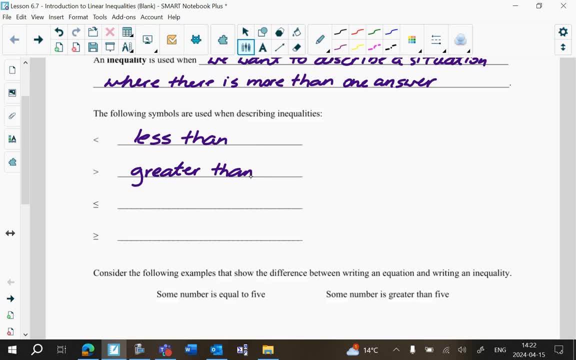 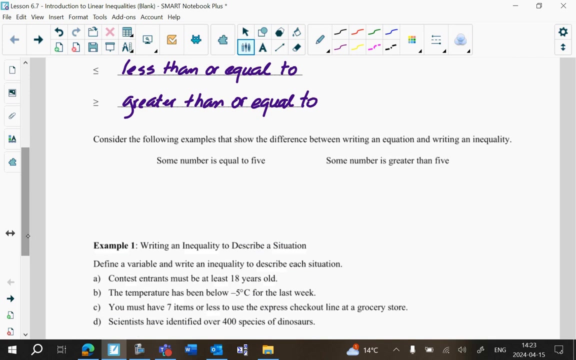 you may just be able to figure it out. you think the next one is less than or equal to its combination and of course, then, if it's going the other way, it would be greater than or equal to. so the big difference, okay, between writing an equation and an inequality, this: 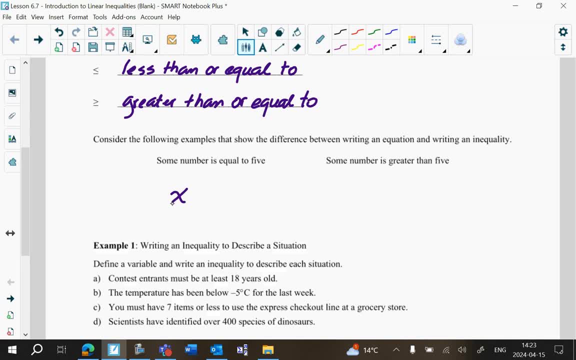 one answer, some number is equal to five. one solution, one solution, this one, some number is greater than five. how many answers spit that? how many possible answers are there? okay, give me a word in math that describes so much. what's that word in that? infinity, infinite solutions, as you can go on and on forever. a lot of. 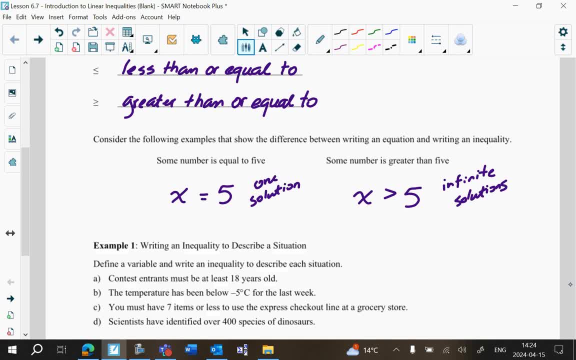 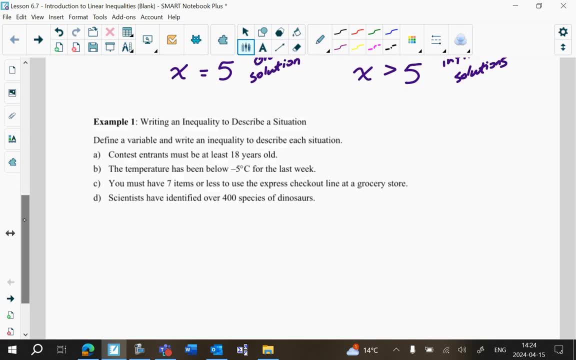 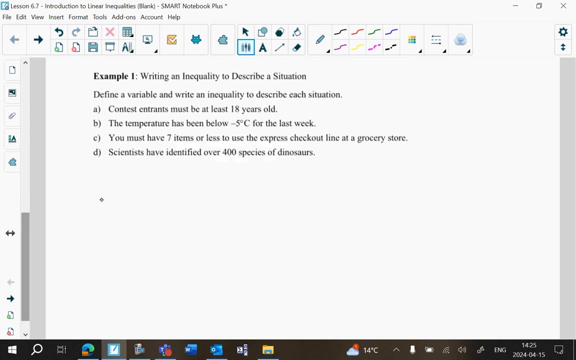 you of inequalities have infinite solutions. okay, so let's just practice using these symbols to each of these sentences to find a variable and make an inequality statement of it. so contest entrance must be at least 18 years old. well, it's the Contest entrance age, So maybe we can use C for contest. 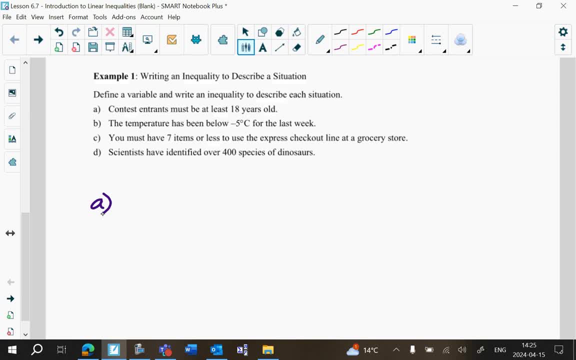 Maybe we can use A for age. What's the rest of the inequality look like? Must be at least 18 years old, At least greater than or equal to. Yeah, I know, when you hear the word least, you think less than. 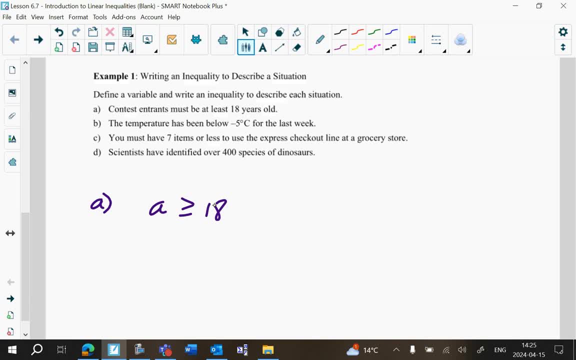 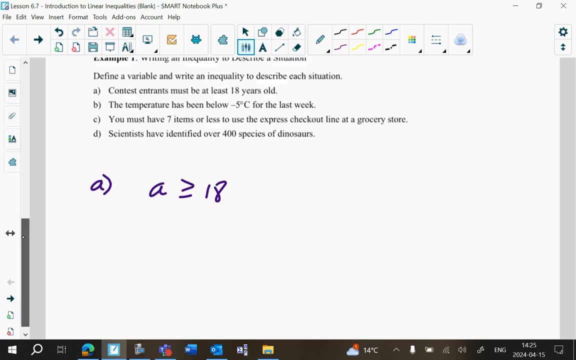 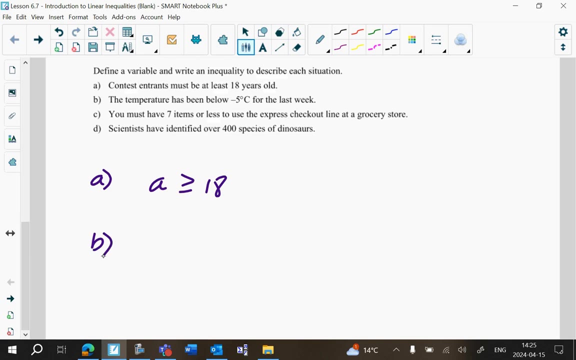 But at least means that amount or bigger, And they can be 18,, which is why we use greater than or equal to. Temperature has been below minus 5 degrees Celsius for the last week. Well, T temperature. How would I finish? 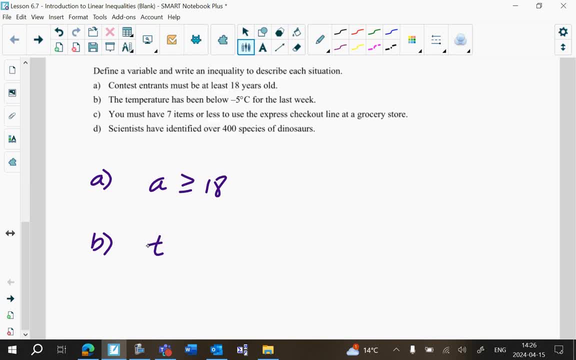 Remember, we don't put units in our equations, They're inequality. We just put the variables, the symbols and the numbers. T Less than. Why do you sound unsure? Okay, Could it be less than or equal to No, because it says less than. 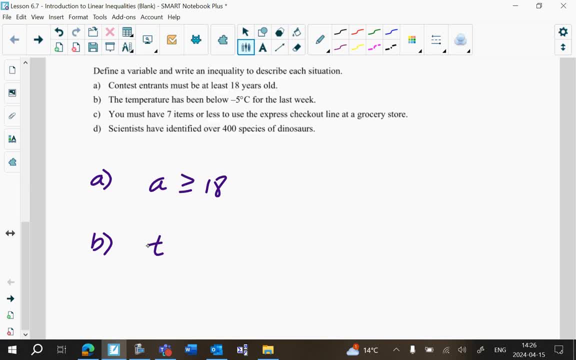 It says below. It doesn't say it's been at or below, So it would be less than minus 5.. You must have seven items or less to use the express checkout line at a grocery store. So items we'll call it I. 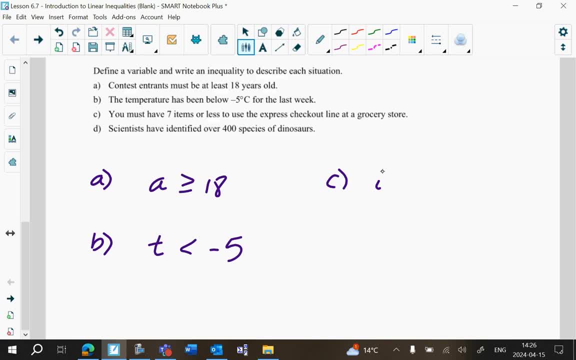 Somebody want to finish it- Less than or equal to Less than or equal to Seven right seven items or less. This one would have several answers, but it wouldn't have infinite answers. okay, Because you couldn't, I mean it would have the only answers. 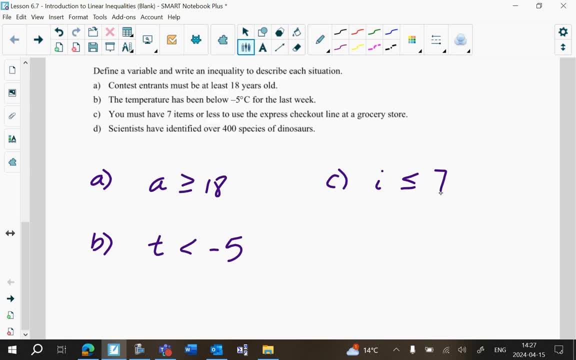 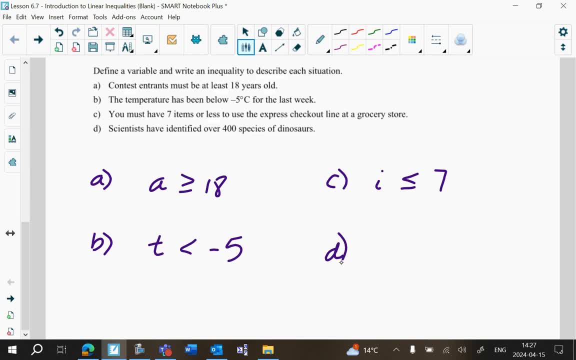 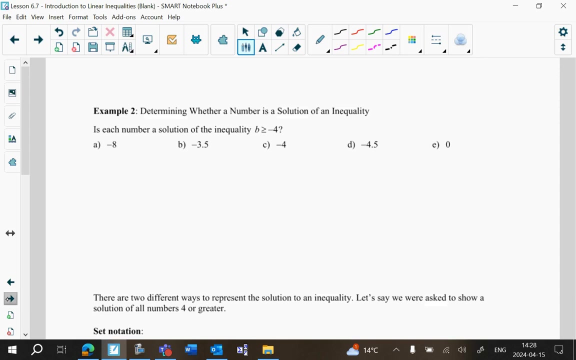 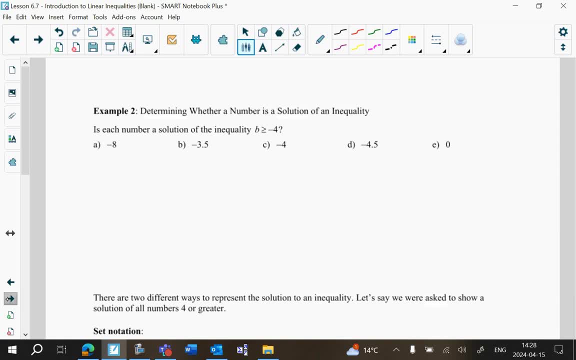 numbers compare to each other, negative numbers compared to positive numbers. so is each number a solution to the inequality. B greater than or negative 4, so is 8 negative. 8 greater than or equal to negative 4. no, is negative 3.5, is negative 4 because that's or equal to, is negative 4.5 and is 0. there we go. 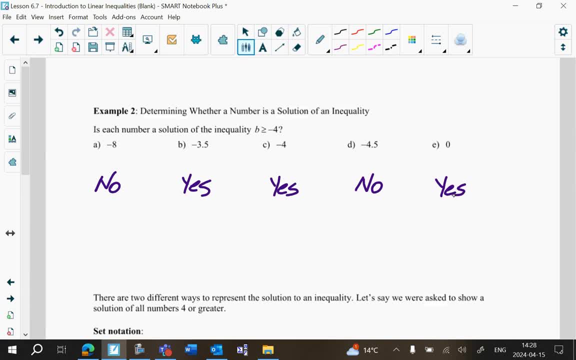 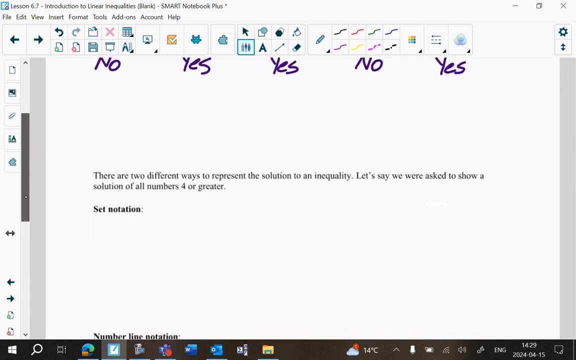 okay. okay, there's a few different ways that we can show inequalities. the most common way is using those inequality symbols, a variable and some numbers, but many times we can show it graphically as well. and how do we show it graphically? we use a number line. so 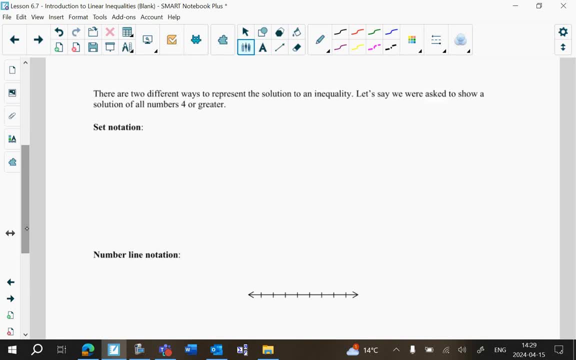 the two ways that we're going to talk about. there is a third way that we'll talk about next year. okay, let's say we're asked to show a solution of all numbers for a greater step. notation uses variables, you, you, inequality, signs and numbers. it's what we've just been doing. so if I want to show X or, sorry, if I want to, 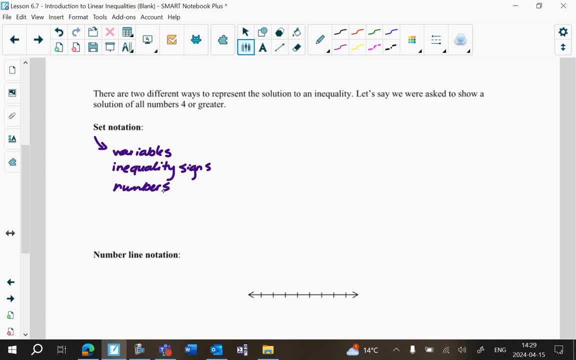 show every number greater than 4 or equal to. I would just go 8 X greater than or equal to, negative you, if I want to show it using a number line. well, what I usually do with a number line is: I put two points of reference on. 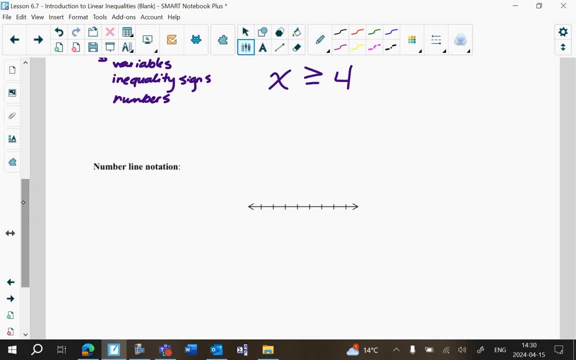 the number that I'm asked, or the number that's at the inequality symbol: either greater than, less than, greater than, or equal to, less than, or equal to, and 0. okay, so if I put, say, 0 here, then 4 is going to be 1, 2, 3, 4 here. 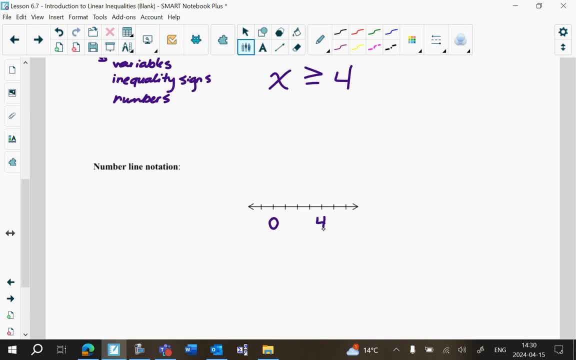 because everything's happening. that's 4, okay, so I started 4 and I go larger. how do you think I could show larger on a number line? how do you think I could draw bigger? what could I draw? any idea. I want to show bigger when I move to the. 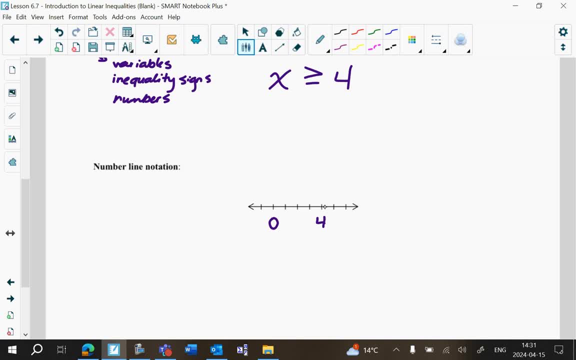 left or right to the right because it's bigger right. so what I would do is I draw an arrow like that that shows everything bigger than 4, but I haven't addressed 4 yet. do I include 4 or do I not include 4? I do so when you include the number at the. 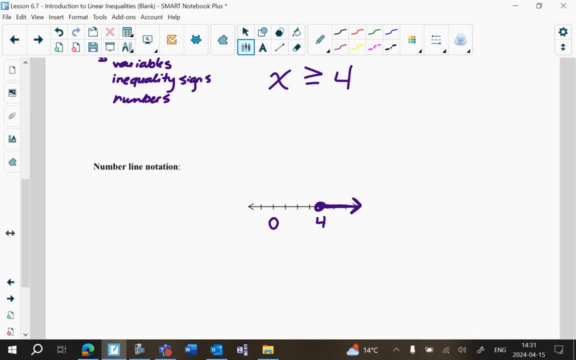 inequality. you put a filled in circle or we call it a closed circle. if we didn't include it, we would put an open circle or a hollow circle. that means we started 4 but we don't include 4, and then we go out to the right. so when 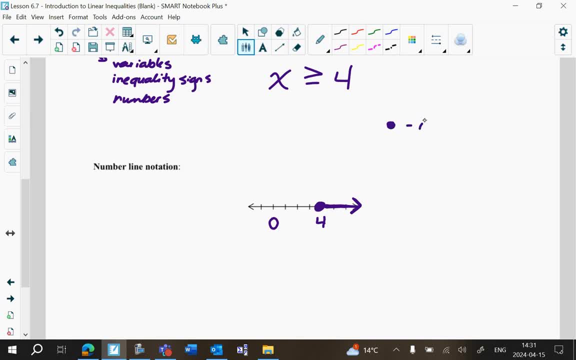 you've got a dot like this, this means include. when you've got an open circle like this or a hollow circle, don't include, and we'll practice with a few of them right now. so here we have a bunch of inequalities and we're asked to graph, so what we want. 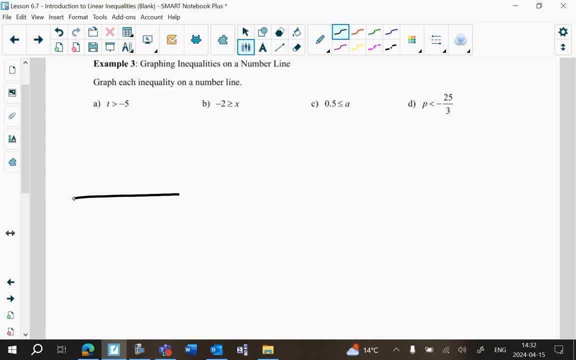 to do. you don't have to put out, you don't have to draw a whole bunch of notches. it's happy things are happening. at negative 5. put that on your number line and put 0. so how would I put negative 5 and 0 on? well, negative 5 is to the left. 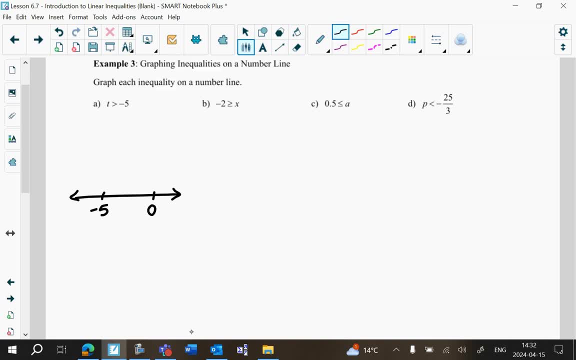 of 0, so you just have to do that. you don't have to put the notches in between. and then how would I show everything greater than negative 5? what kind of circle would I put it? negative 5, negative 5, hollow or open? because I'm not. 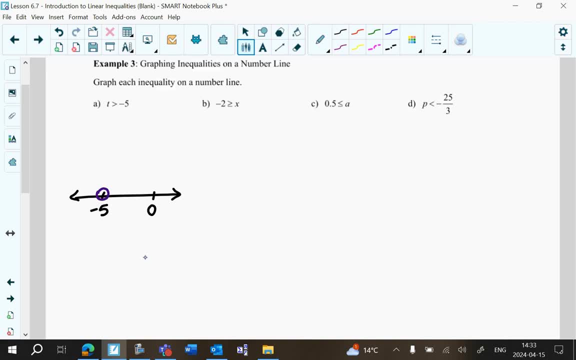 including it now. does my arrow go off to the right or left so looks like that. don't get thrown by the second one. it's just written in a different order. write it back in the same. write it back with the variable first. if negative 2 is. 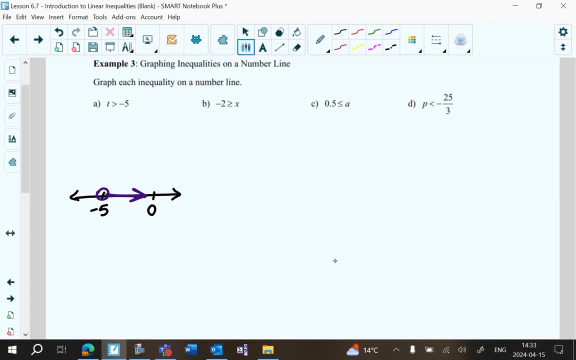 is greater than or equal to x, then working backwards x is- remember I'm going backwards- less than or equal to negative 2. and then do that one. so we would draw a number line, two notches: 0 goes to the right because it's bigger than negative 2. and then how about I draw my circle and my arrow? 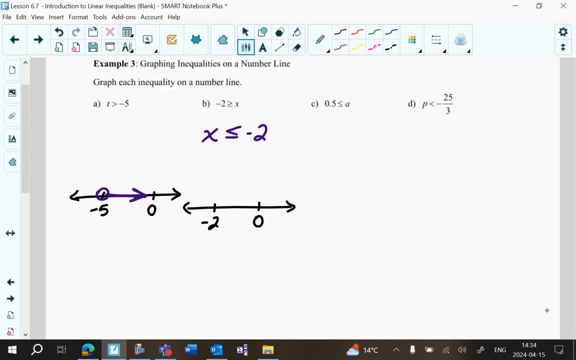 going to the right, going to the left, and what kind of circle at negative, 2 filled in- and going to the left. yes, that's what it would look like. again. if it's backwards, just write it the other way around. it's: 0.5 is less. 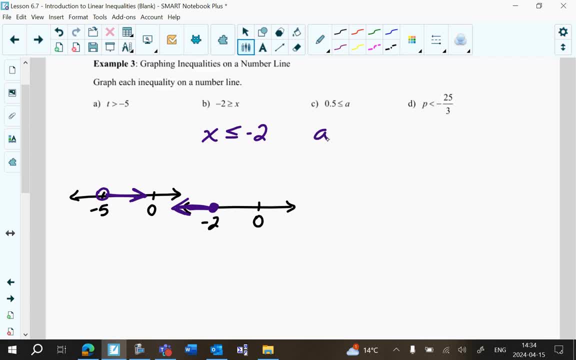 than or equal to a. that means a must be greater than or equal to 0.5. draw your number line, put your two point. put your two notches. one for 0, 1, 4.5. this time 0 goes on the left because 0.5 is bigger. 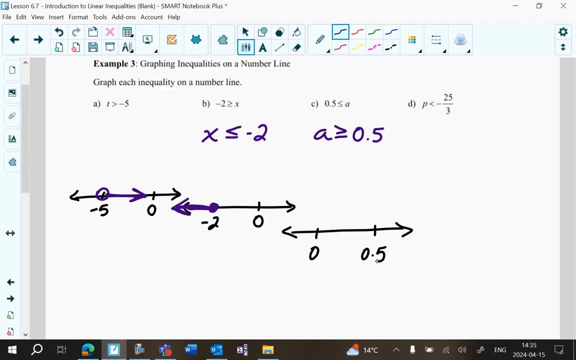 what kind of circle at 0.5 filled in or closed, and my arrow goes off to the it's greater than or equal to 0.5. yeah, that's one way to look at it. this is the way that the inequality symbols point is. the same way the arrows. 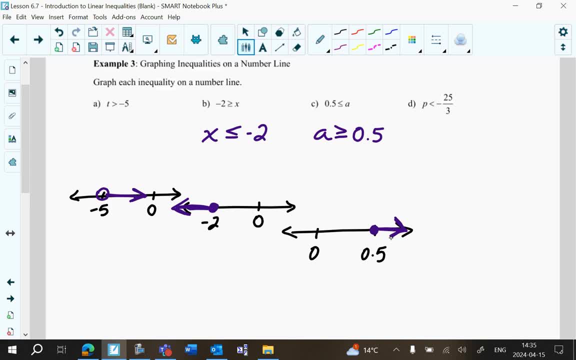 point. and finally, this last one, don't get thrown by the negative fraction, and it's negative, so I know it's going to go somewhere to the left of 0 and I just want to show less than that value. so what would I put at negative 25 over 3, all over open circle? and then I would 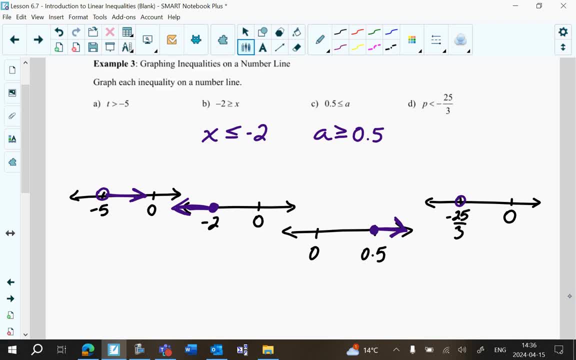 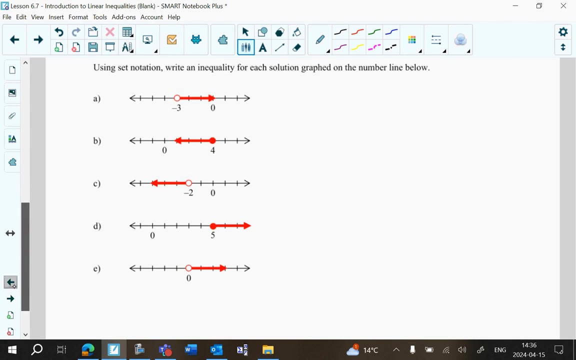 go to the left. okay, so that's going from set notation graphing line notation. what if we go the other way? I give you the graphing line notation, you tell me the set notation and they're all going to begin with X or whatever variable you choose. you don't have to. 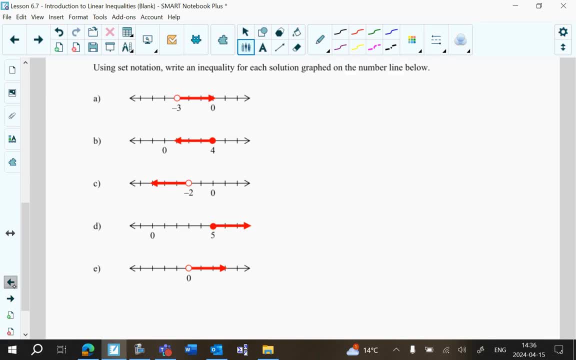 choose X, and then some inequality symbol, then some number. so what would the first one be? X, you, no, you could do the number first if you wanted, to less than greater, to greater, to greater than, why not greater than or equal to the thing circles a, hollow circles a. 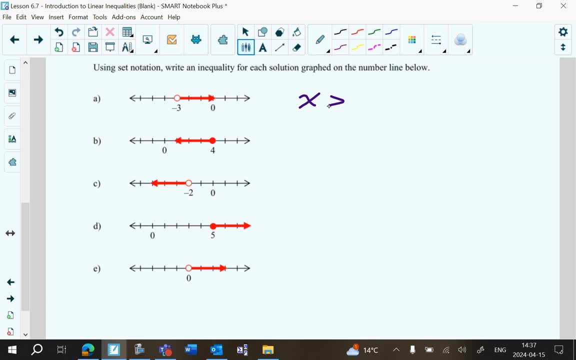 hollow circle. yes, that's what you said before. yeah, I'm just messing with you. then you've got to come back tonight, where's math is a bad thing. thank you so much. what do you know what, Matty? I have one question. what do you hurt yourself? 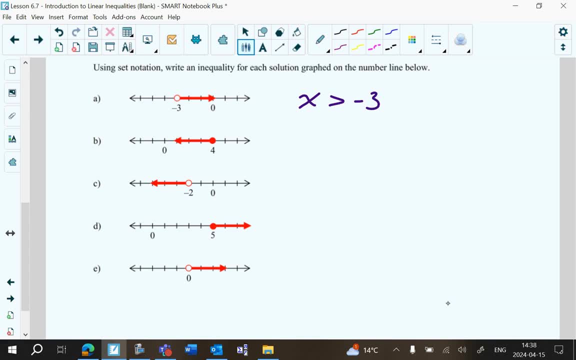 why must you hurt me? one must you hurt me? you know how sensitive I am. I'm a very sensitive fellow and I have to go all the way down to the first floor because that's the only place where a men's washroom is. if I want to go cry because I'm so sensitive, yeah, but 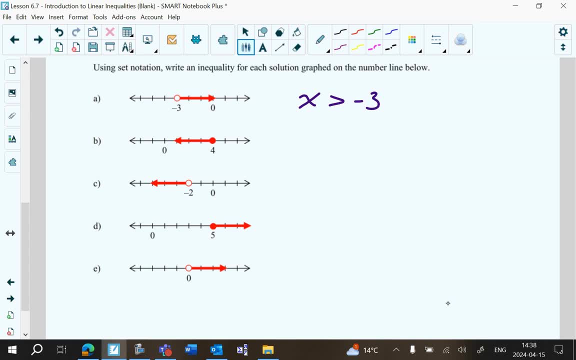 if I make you cry, you only have to go there. you make me cry. I have to go down two flights. yeah, see now. why not again? why hurt me? why are you hurting me? because I come after you. I'm an angel. I've said nothing but nice things to you.